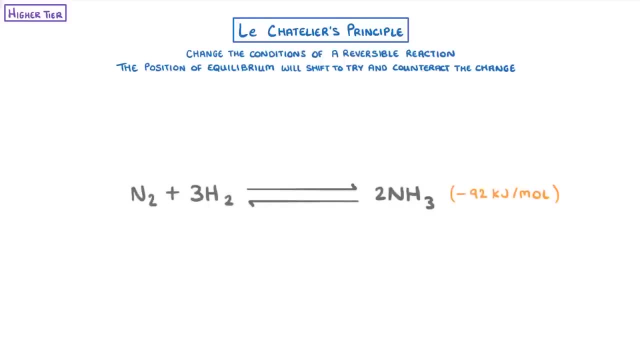 To see what this means in practice, let's take a look at the following example. Let's take a look at this reaction for the production of ammonia from nitrogen and hydrogen And imagine that it was being done within a sealed system. The minus 92 kilojoules per mole is the overall energy change of the forward reaction. 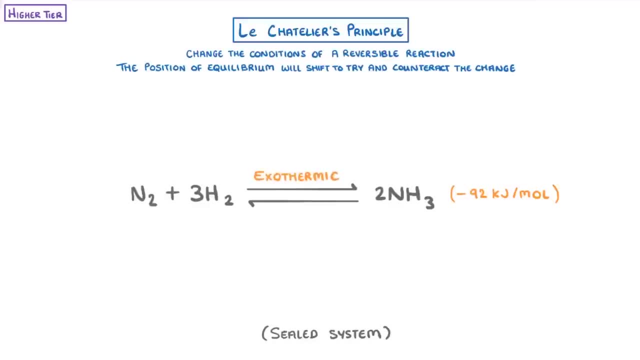 And because it's negative, we can tell that the forward reaction is exothermic, which means it releases energy to the surroundings. And because the backward reaction has to be the opposite of the forward reaction, it must be endothermic. For the sake of our example, let's imagine that the position of equilibrium starts off. 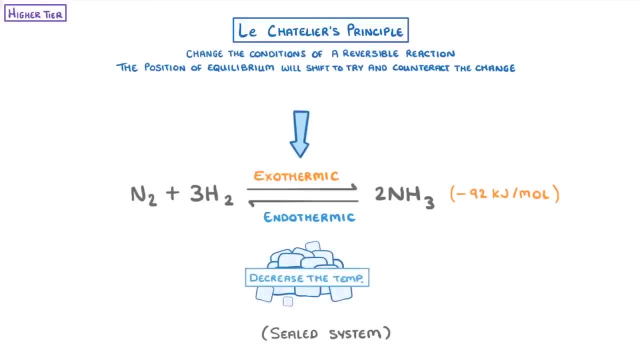 here in the middle. If we were to decrease the temperature of our system, the equilibrium would move in the exothermic direction in order to release heat energy and counteract that change that we just made. In this case, that would mean the position of equilibrium moves to the right, so it would. 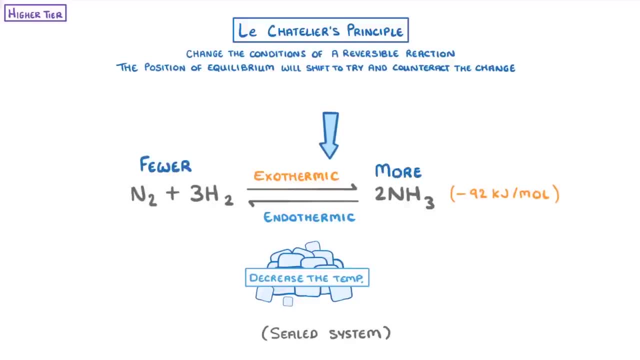 have more ammonia particles and fewer nitrogen and hydrogen particles. On the other hand, if we increase the temperature of our system, then to oppose this change and decrease the temperature, the equilibrium would move in the endothermic direction, so to the left. 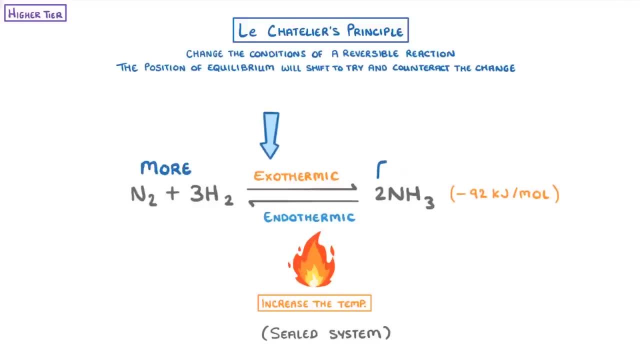 Which means we'd have more nitrogen and hydrogen but fewer particles of ammonia. We can also apply this concept to the pressure of our sealed system. So if we increased the pressure of our sealed system, we would have more nitrogen and hydrogen but fewer particles of ammonia. 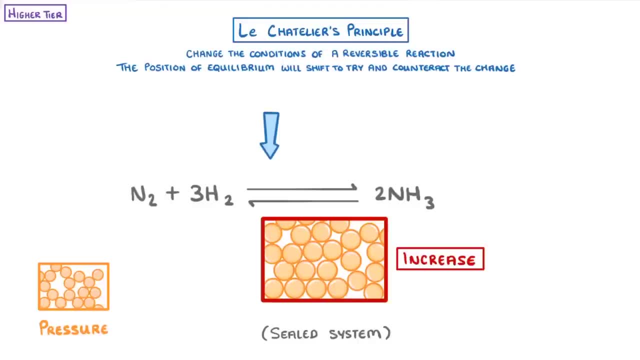 And if we increased the pressure, then the equilibrium would move to whichever side reduces the pressure back down And as pressure is basically just a measure of how many particles there are per unit of volume to lower the pressure, the equilibrium would move to the side with the least number. 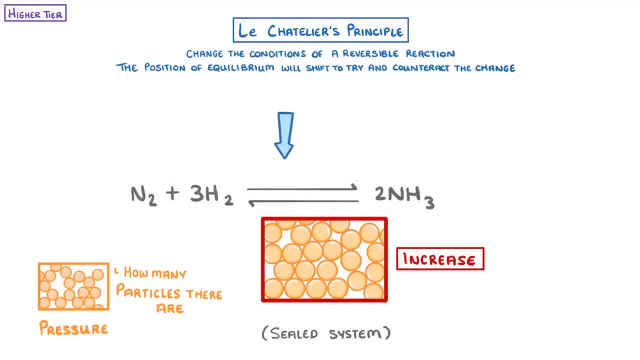 of molecules, which, in this case, is the right because there are only two molecules of ammonia on the right hand side, whereas there's four molecules on the left, because there's one nitrogen plus three hydrogens. On the other hand, if we decrease the pressure, then the equilibrium would shift to the side.